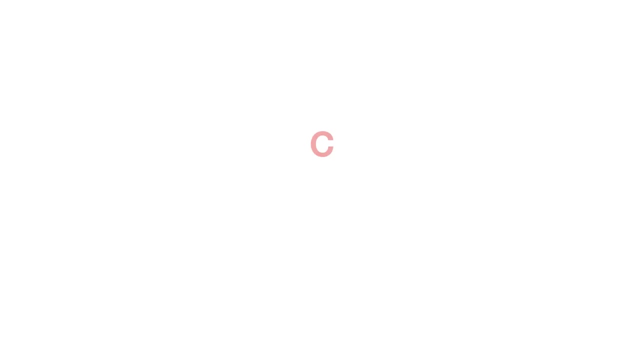 Nuclear Facilities are based on what is referred to as the Pickering Nuclear Generating Station: Control, Cool and Contain. For all activities, priority is given to ensuring that at all times, the reactor power is controlled, that the fuel is cooled and that the radiation. 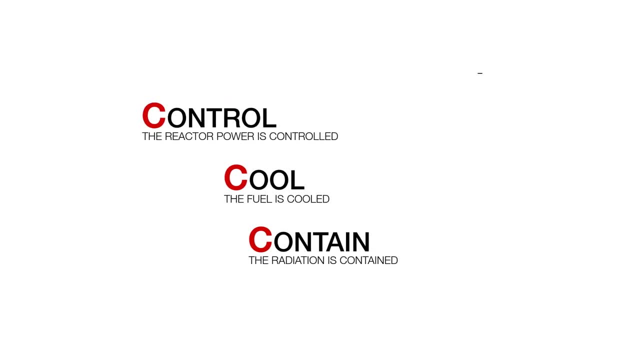 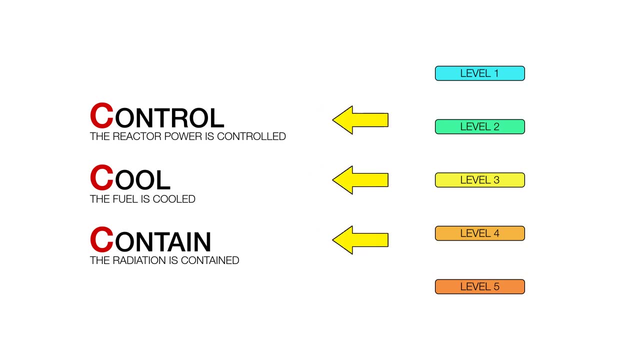 is contained Supporting the three Cs principle are five levels of defense which ensure that multiple, independent and diverse barriers are maintained to protect the three Cs at all times. The five levels of defense assure that the likelihood of accidents are minimized and that the resulting likelihood of a large radiological release is extremely small. 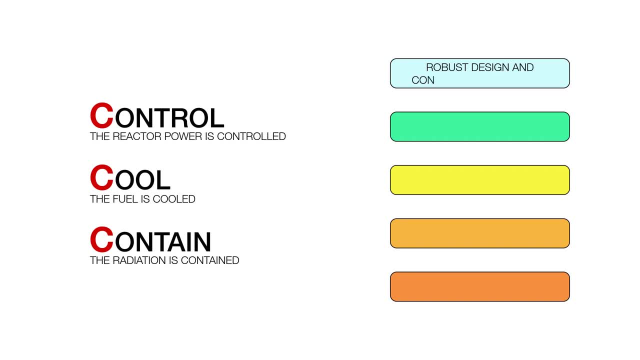 Pickering's five levels of defenses are: Robust design and conservative operation. Reliable process systems. Multi-groups of engineered safety systems. Flexible emergency mitigation equipment. Comprehensive emergency preparedness plans. The following illustrates how Control, Cool and Contain function and the robustness of Pickering's design, which is the first level of defense. 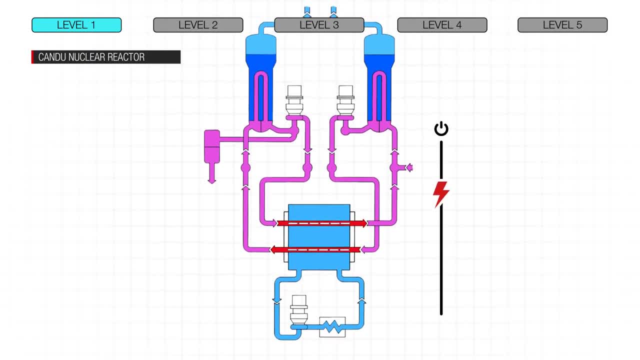 Control, Cool and Contain. If an event occurs where it is required, reactor power is automatically reduced and the reactor is shut down. This is the first C Control. Although the reactor is shut down, the fuel in the reactor continues to generate. 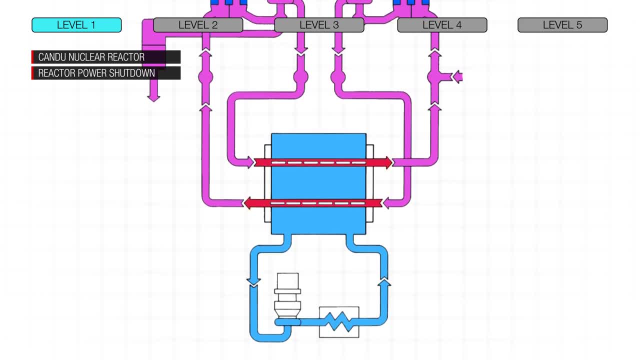 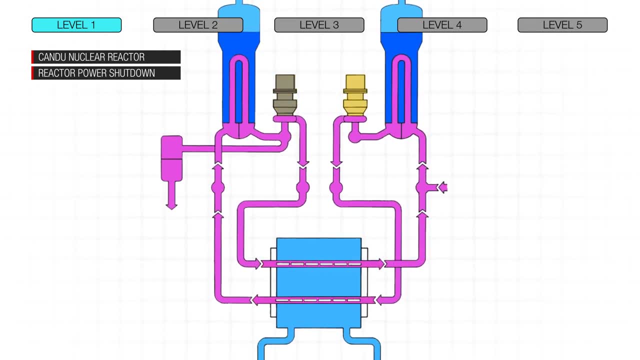 a small amount of heat, so the fuel is continuously cooled. Like all other nuclear power plants, Pickering's normal process systems are capable of cooling the reactor If normal cooling is interrupted- a unique and reliable design feature of all can-do stations, called natural. 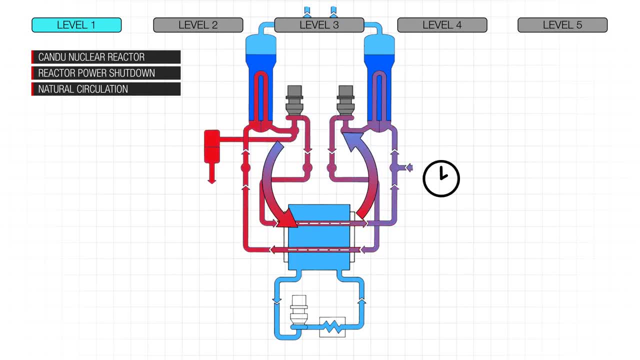 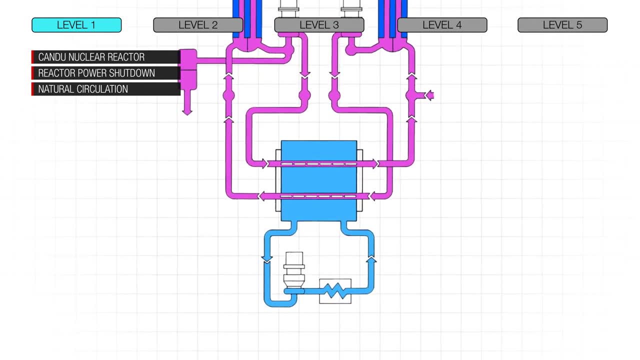 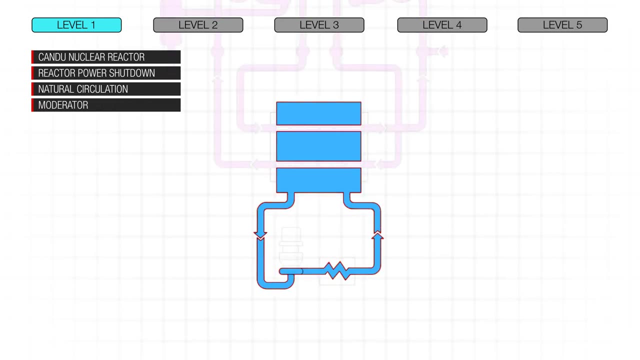 circulation will continue to cool the fuel. Natural circulation provides enough time for normal power to be restored or an alternative means of cooling to be established. Another important feature of the can-do design is the ability to cool the reactor using the very large inventory of water in the moderator tank In the unlikely event that natural circulation 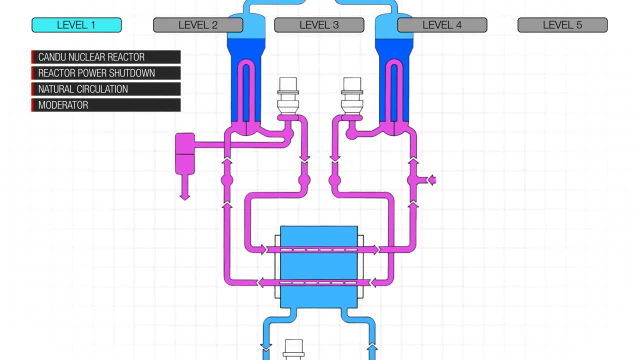 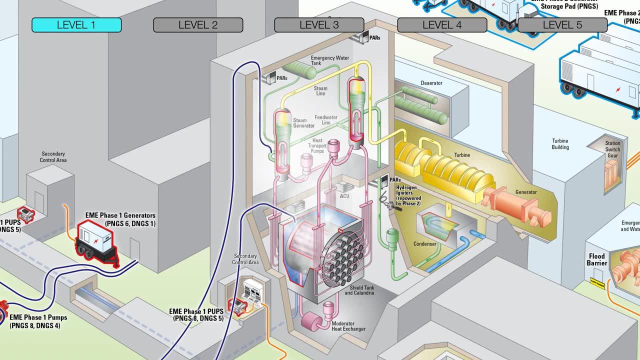 fails. maintaining the moderator tank filled and continuously replenished with water will keep the reactor cool. Any steam that is created from fuel cooling that may be released to the reactor building is managed by air conditioning units. The ACUs cool and condense the steam. 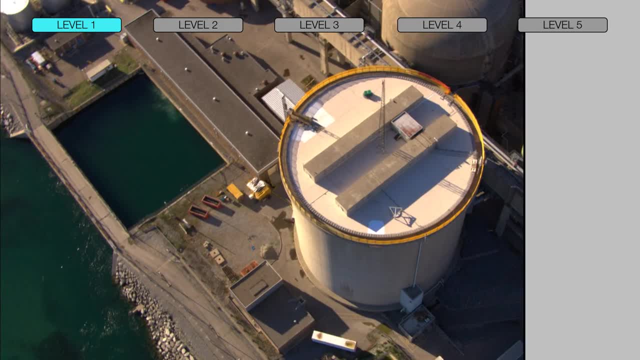 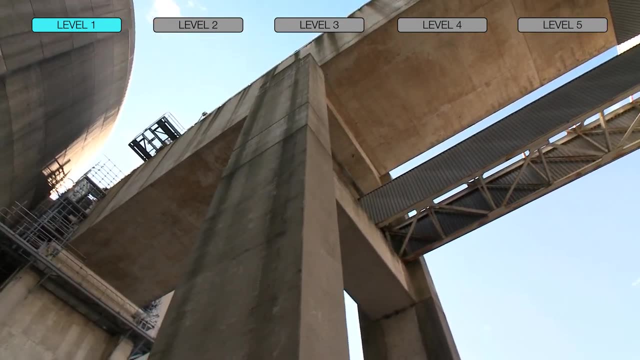 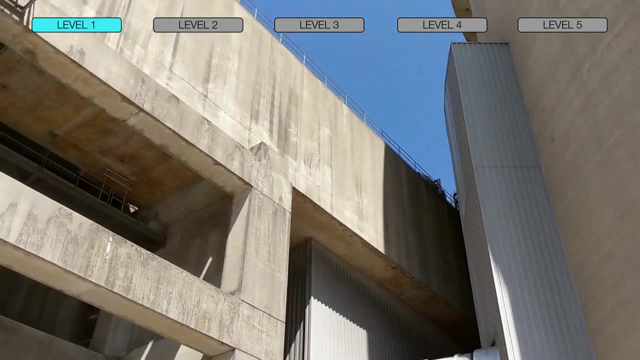 and thereby reduces pressure within containment. The Pickering vacuum building, another important design feature for all multi-unit can-do stations, is also available to condense and contain any steam. The Pickering containment system minimizes radiological releases by virtue of its very large volume, thick concrete structure and maintained at negative pressure by the 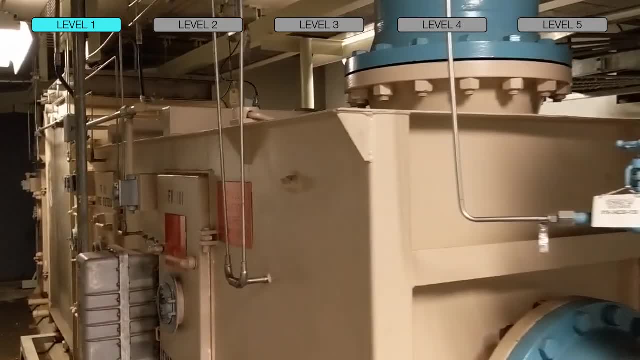 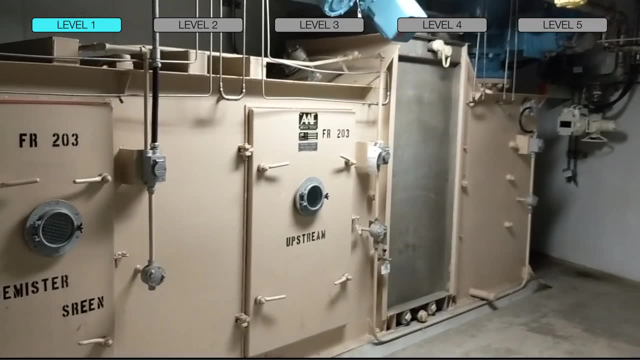 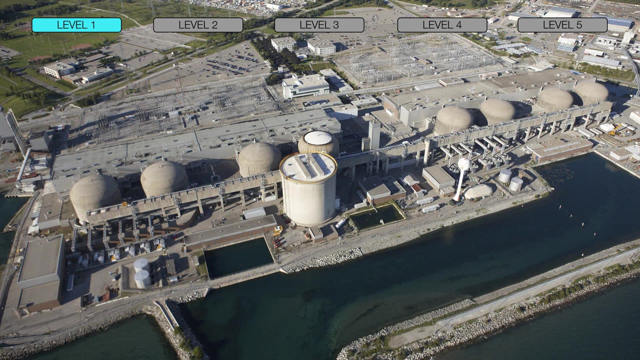 vacuum building To control containment pressure. in the longer term, a filtered air discharge system comprised of high-efficiency filters can be used for controlled filtered venting. To illustrate how the three Cs are protected by the multiple levels of defense, consider a station event where there is a total sustained loss of all off-site electrical power. 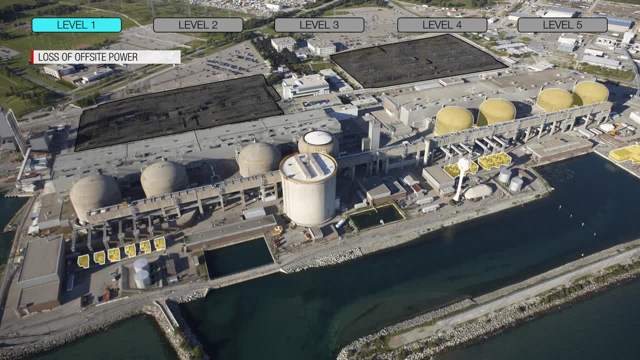 The Pickering station has multiple diverse and independent sources of on-site electrical power that prevent the loss of off-site power from progressing to a total station blackout. If power from the electrical grid becomes unavailable, selected Pickering units will continue to power the reliable station process systems automatically. These systems are the: 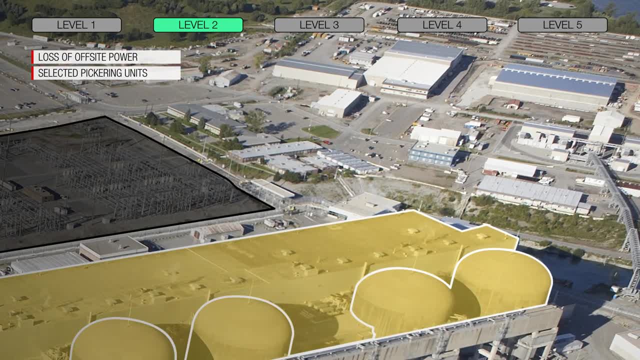 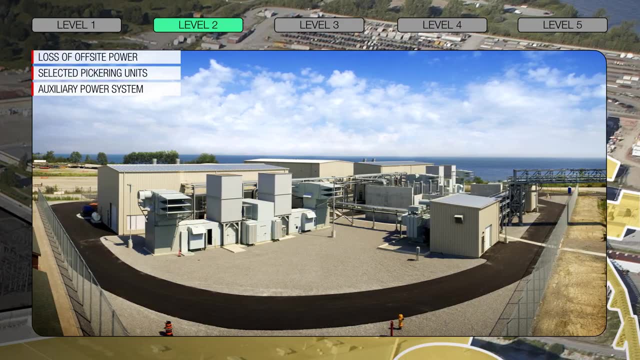 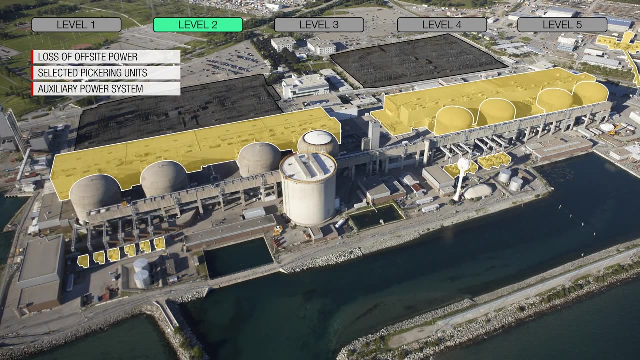 second level of defense. Also available is the auxiliary power system that is comprised of two redundant jet engine power generators that can power the station process systems With electrical loads being supplied by a Pickering unit or the auxiliary power system, Pickering's process systems. 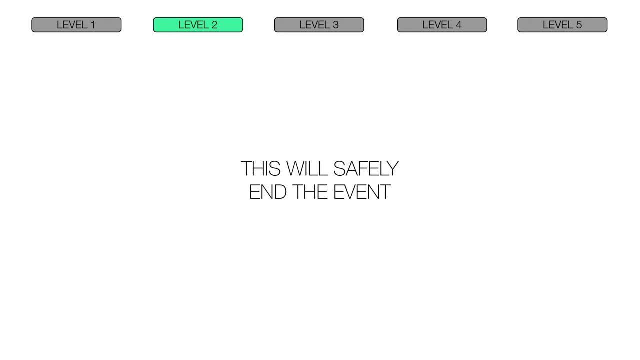 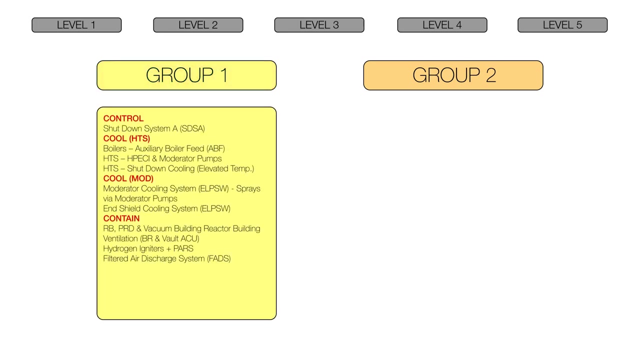 will ensure that the three Cs are maintained. This will safely end the event. Like all other can-do stations, Pickering has two groups of diverse engineered safety systems that can each protect the three Cs independently. Pickering A units were originally designed with one group of engineered safety systems. 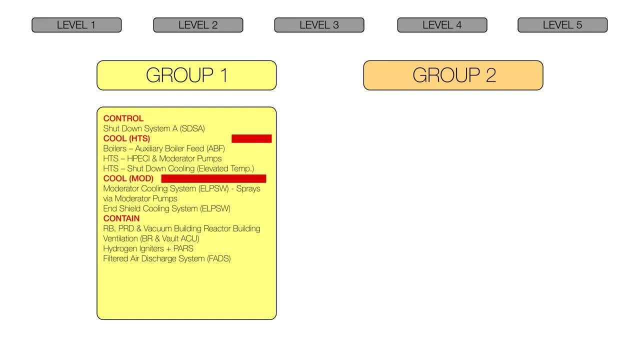 which ensure that the reactor power is controlled, the fuel is cooled and the radiation is contained. Since its initial operation, Pickering A has been modernized to have an equivalent second group, which are additional, independent and diverse engineered safety systems. Pickering A units were originally designed with one group of engineered safety systems. 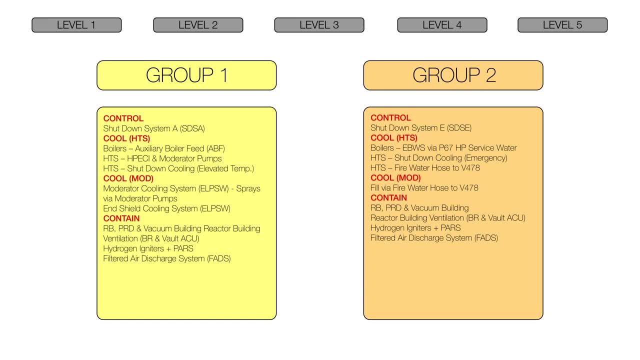 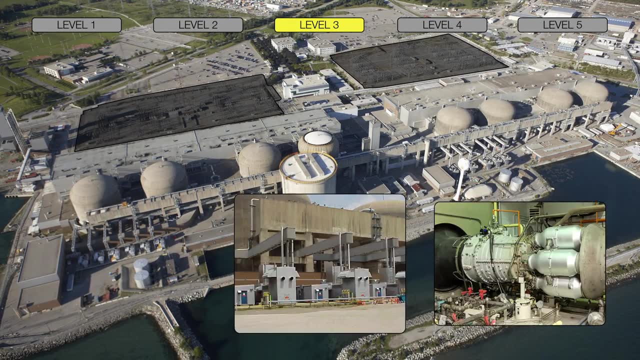 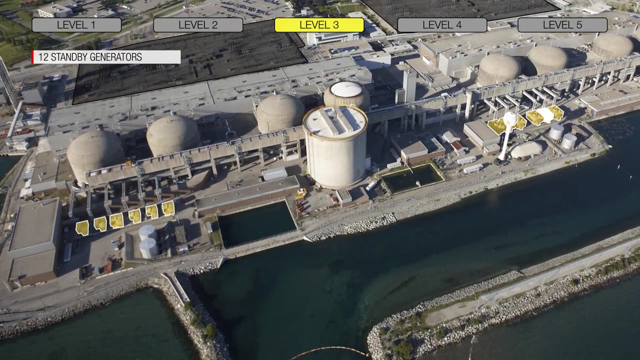 to further protect the three Cs. These two groups of safety systems are the third level of defense. The primary group of safety systems are automatically powered by standby generators upon loss of the electrical grid. There are twelve standby generators at Pickering, of which only four are required to power the 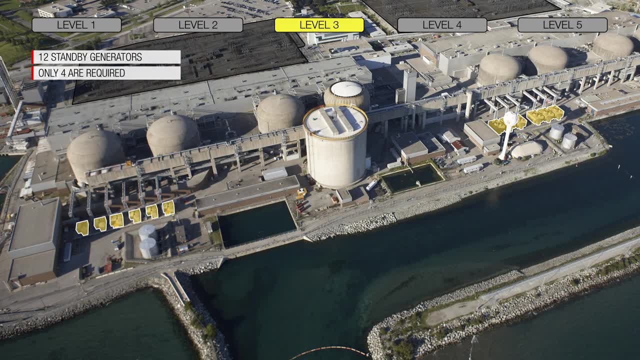 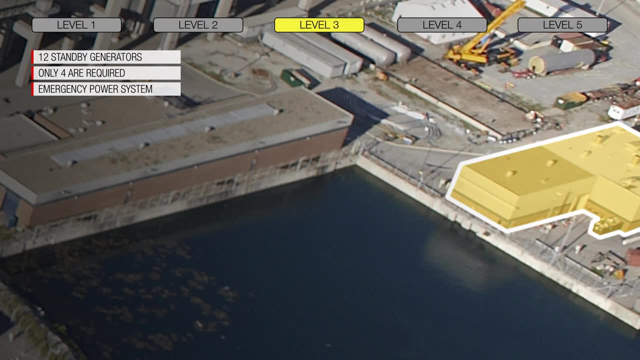 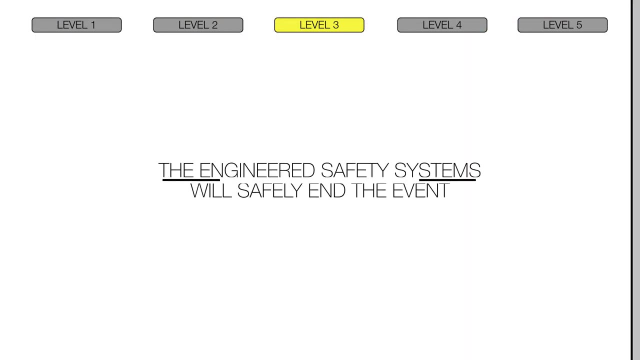 safety systems and assure that the three Cs are maintained. An independent, diverse and seismically qualified secondary group of safety systems are also available to protect the three Cs. This secondary group of systems are powered by the emergency power generators and select standby generators. 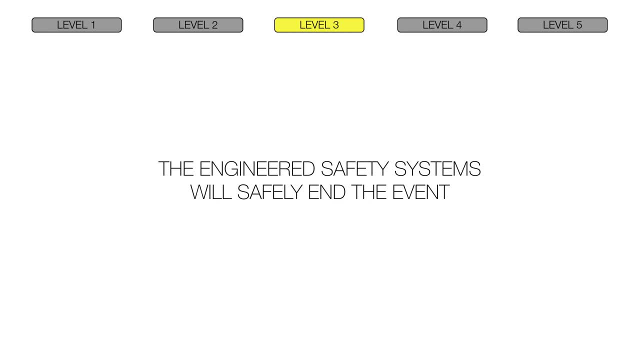 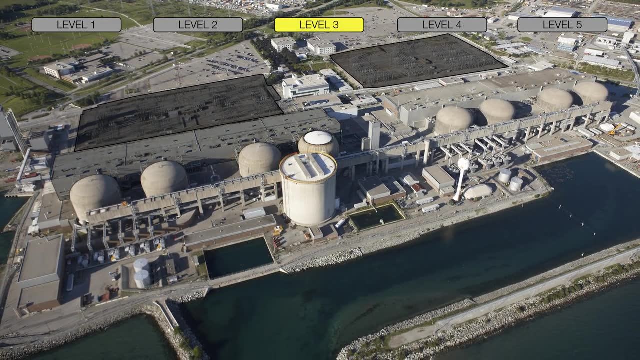 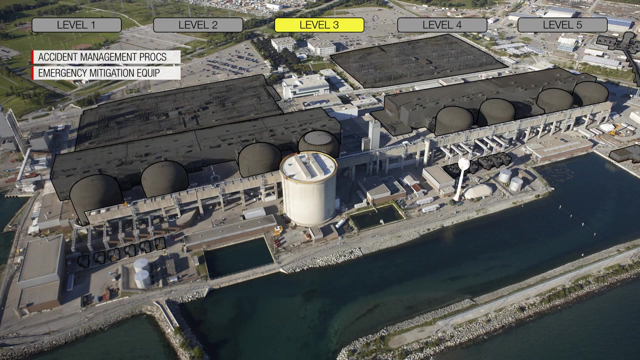 Successful operation of either group of the engineered safety systems will safely end the event and prevent a large radiological release, Although it is very unlikely. should the engineered safety systems fail to end the event, Pickering has in place severe accident management procedures and supporting flexible emergency mitigation. 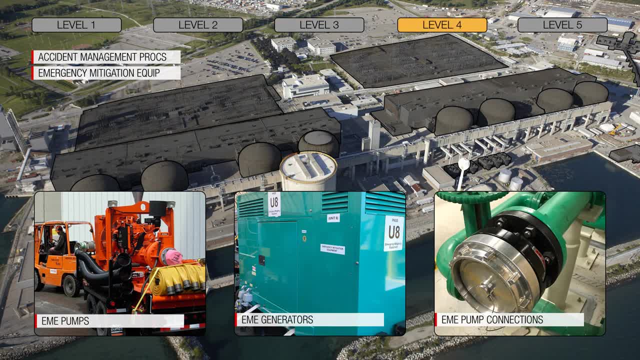 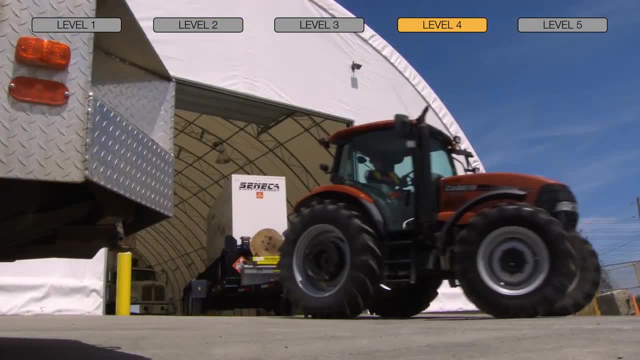 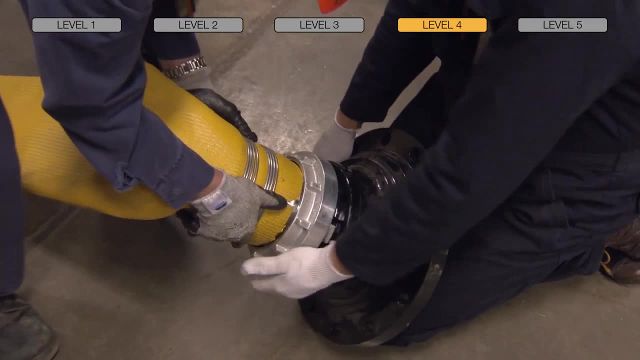 equipment. This is the fourth level of defense that has been significantly enhanced following the lessons learned of the Fukushima event. The equipment consists of portable diesel-powered generators and pumps that allow the repowering of essential station systems and cooling water addition through permanently installed quick connections. 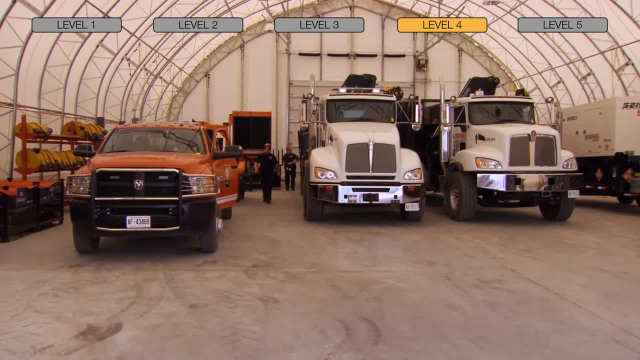 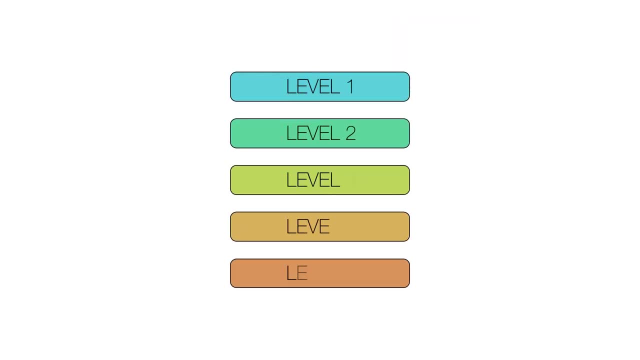 With the successful protection of the three Cs being achieved through emergency mitigation equipment, the event is safely ended and the large radiological releases are prevented. For a complete station blackout and a resulting large radiological release to occur, all the previous four levels of safety systems will have to be replaced. 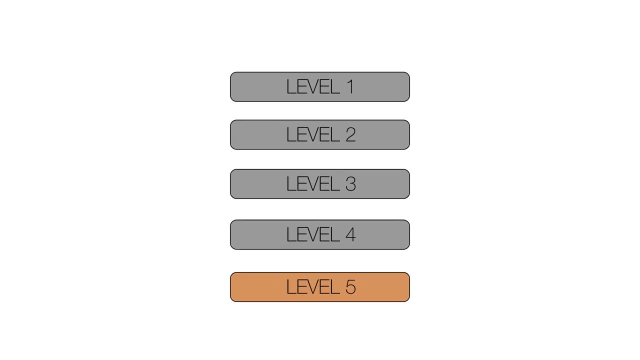 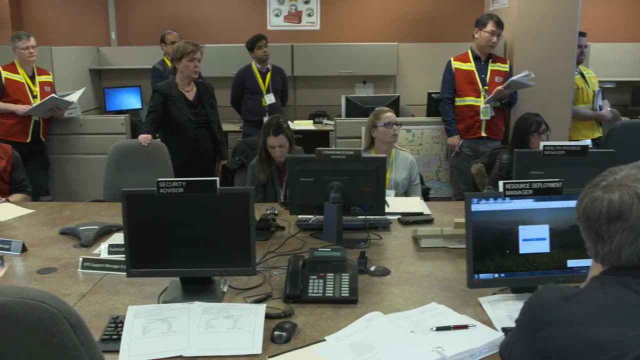 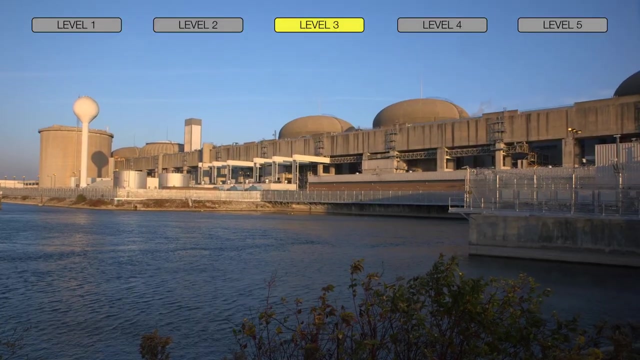 Although Pickering has an excellent safety record and the risk of a large radiological release is already extremely low, further safety enhancements are committed in the Periodic Safety Review Integrated Implementation Plan. The cooling capabilities of the third level of defense at Units 1 and 4 are being strengthened. 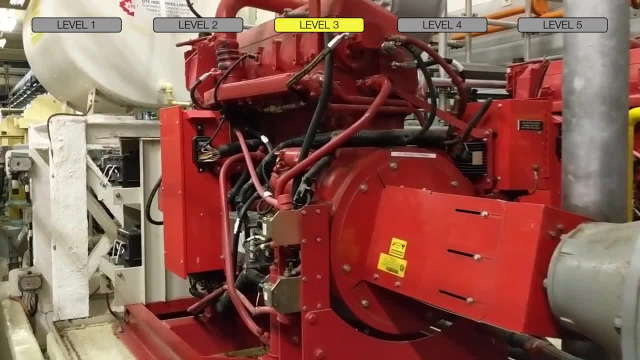 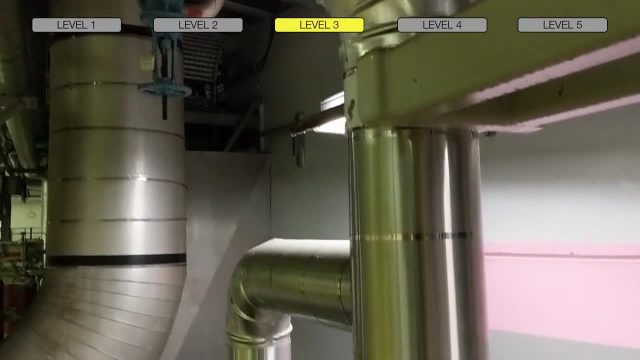 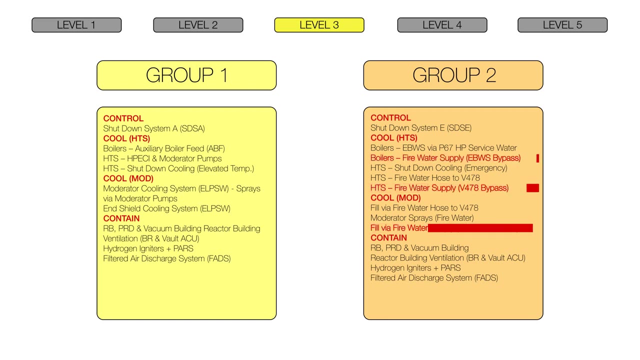 A new plant modification is being made that will allow the use of existing diesel firewater pumps to provide additional backup cooling water. The diesel fire pumps would be unaffected by losses of both off-site and on-site electrical power. The above modifications further bolsters defense in-depth and practically eliminates the likelihood. 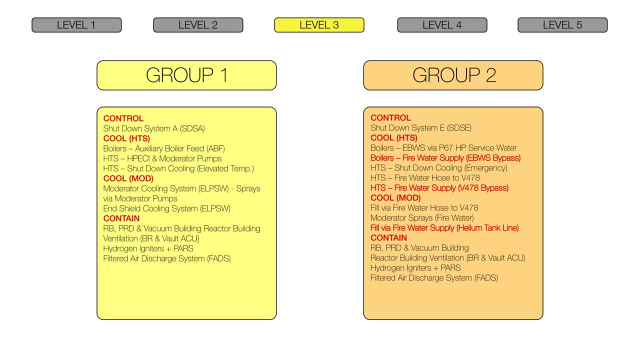 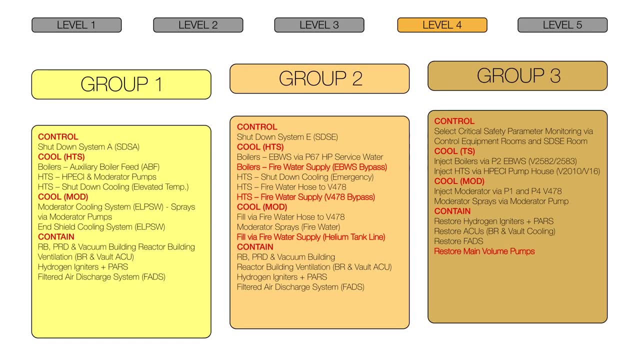 of a severe accident progressing beyond the capabilities of the third level of defense Pickering will also enhance the reliability of the EME function that supports controlled filtered venting. When these modifications are factored into the Probabilistic Safety Assessment, the EME.